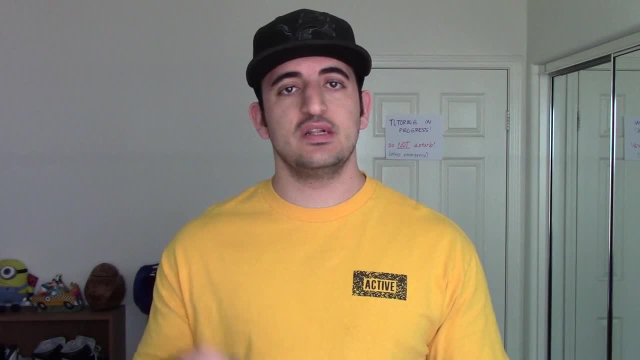 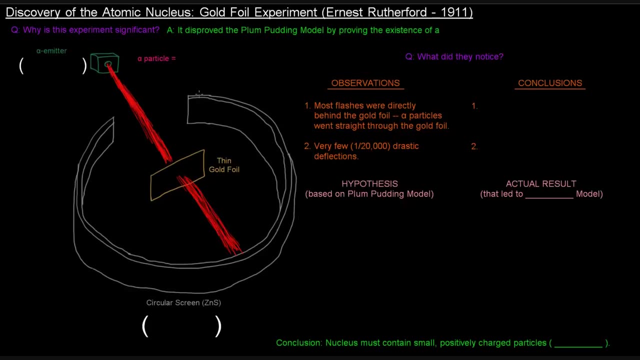 Support MOVE University in the production of more videos by visiting the link in the description below, where you'll find more details. Thank you and enjoy. Next up is the Gold Foil Experiment by Ernest Rutherford in 1911, where he discovered the atomic nucleus. 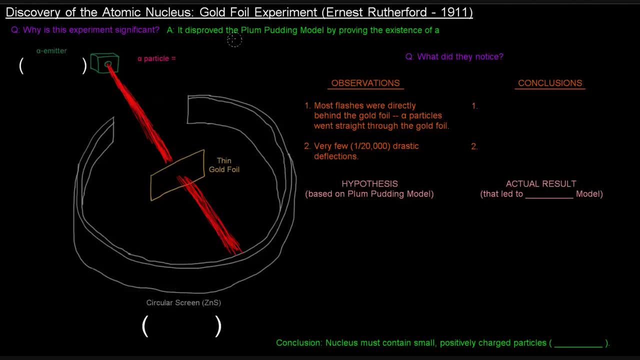 His experiment was pretty significant because it disproved the plum pudding model by proving the existence of a small, dense, positively charged nucleus at the center of the atom. So how did he do that, What was his sort of setup and how did he observe and conclude all that he concluded? 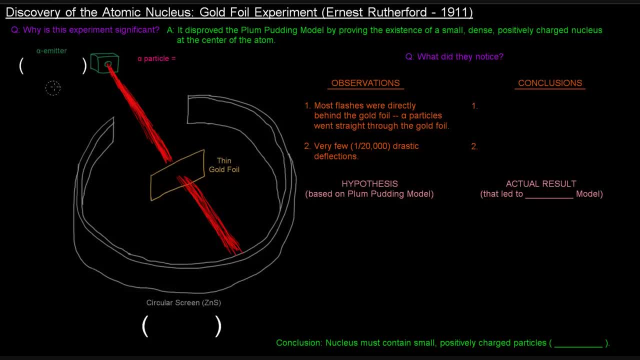 Well, he set up this apparatus that had an alpha emitter which shot alpha particles at a thin strip of gold foil. It shot at a thin strip of gold foil and around this gold foil was this circular screen that would basically detect the alpha particles. 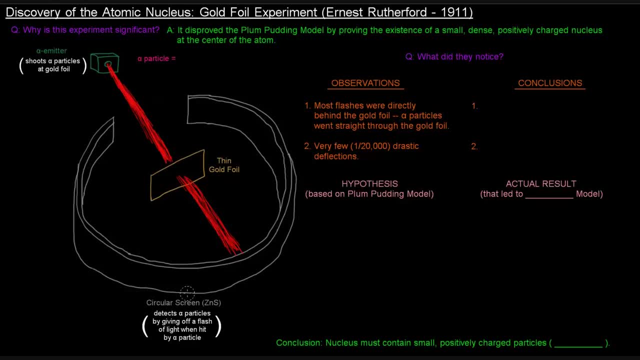 by giving off a foil. It was a flash of light when it was hit by that alpha particle. So I've said the word alpha particle, the words alpha particle, a few times now and I haven't really even talked about what it is. 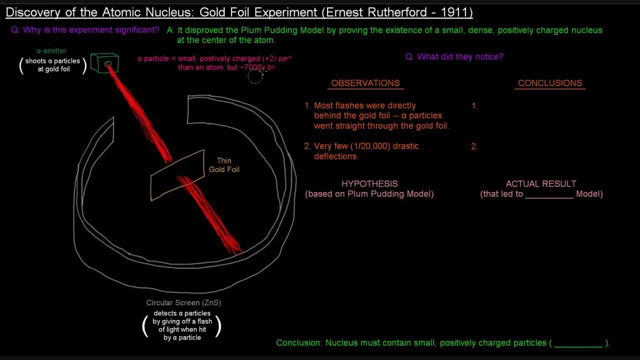 An alpha particle is a small positively charged particle that is much smaller than an atom but 7,000 times bigger than an electron, So an alpha particle specifically have a positive 2 charge. So what happened? was they shot? they took this alpha emitter and it had. it shot alpha particles at this really thin strip of gold foil. 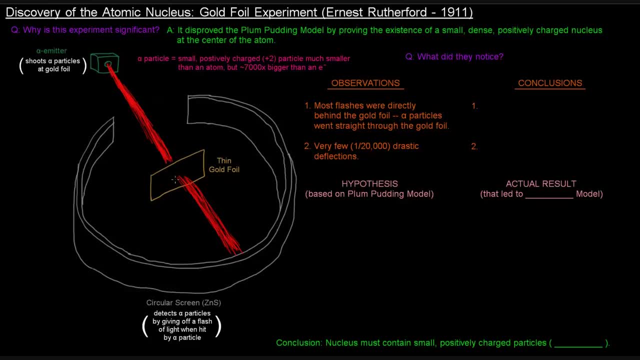 And we want to really know what. what did they notice? what happened? So a lot of the particles went straight through and there was a lot of detection on the screen, right back here, right Tons back here, Tons back here. 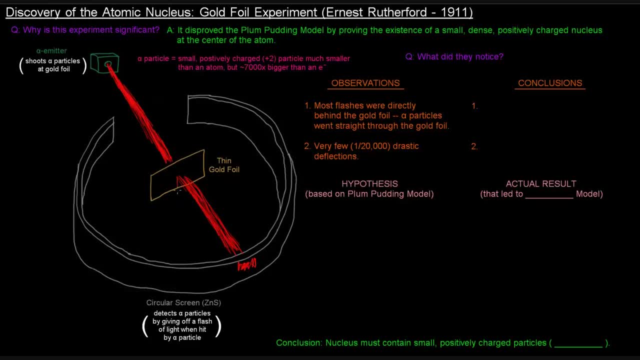 And there were some, some situations in which it lit up over here and and over here. So, and what's kind of crazy is that there were some, some cases in which the detection was over here or even back here. Okay, So they noticed that most of the flashes were directly behind the gold foil, directly behind the gold foil, which meant that 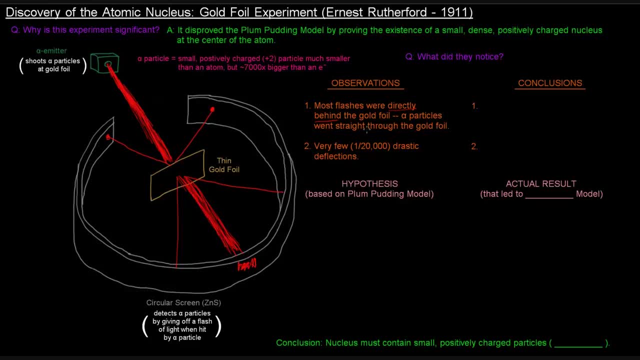 Basically, that alpha particles were going straight through, straight through the gold foil and to the other side. So what did Rutherford conclude based on that observation? Based on that observation, he concluded that the atom is mostly empty space If these particles are just traveling straight through. 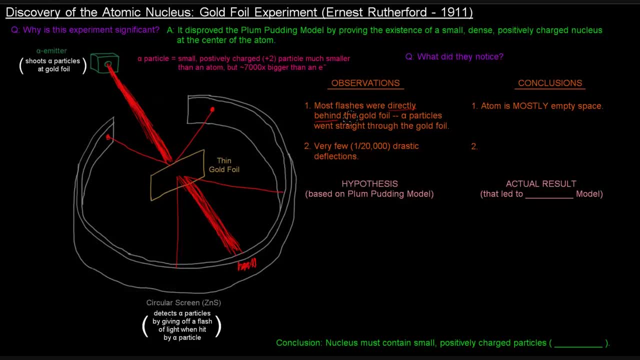 the atom must mostly be empty space. But what he did notice is that there were very few- one in every 20,000, drastic deflections or major deflections. So there were some that might have been pretty minor, where, if you notice, instead of all of them going straight in a straight line, 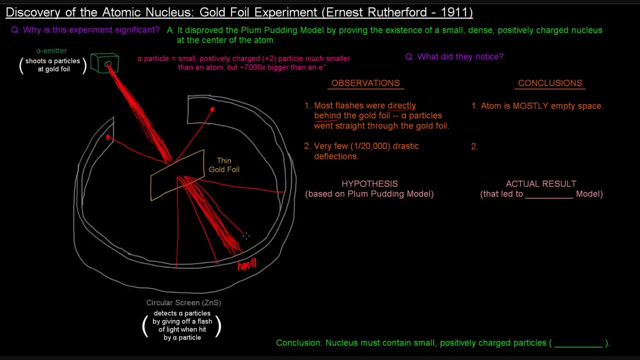 there might have been some that came off like this or like this, But there were some that came pretty much back in the direction where the alpha particles came from. So that was kind of crazy, And so the conclusion that they drew from that was that 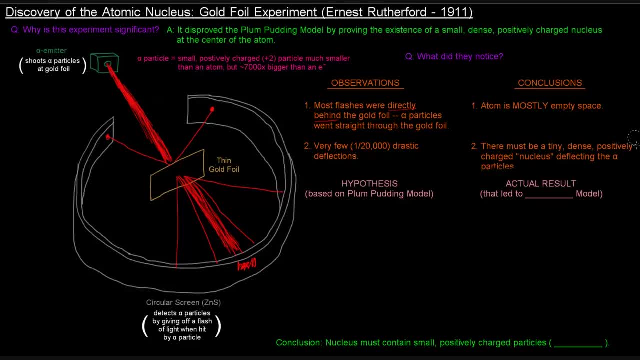 there must be a time, a tiny, dense, positively-charged nucleus deflecting the alpha particles. So let's think about why. this would be the conclusion based on the hypothesis. The hypothesis was based off of the plum pudding model. Okay, the plum pudding model. 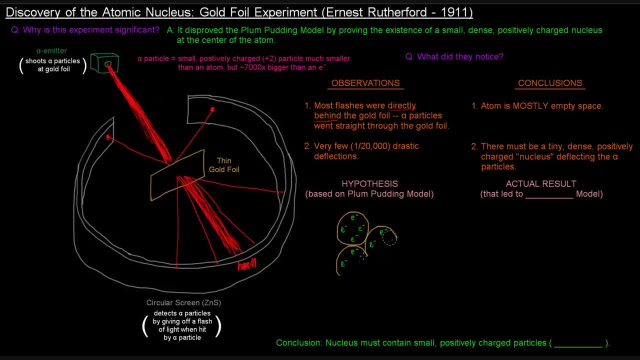 So the plum pudding atoms look like this, right Where they have that positively-charged fluff, the positively-charged fluff and these electrons. So the hypothesis was that if we shoot, if he shoots alpha particles at this thin gold foil. 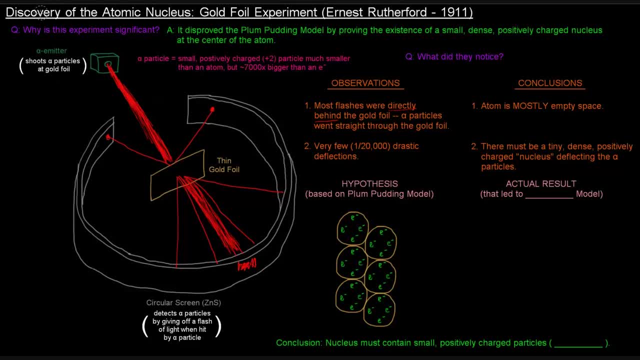 this gold foil was supposed to be a few atoms thick, right? So if we think about these just being the actual gold atoms, sort of aligning themselves like this, shooting these alpha particles at them, if the plum pudding model is the case, right? 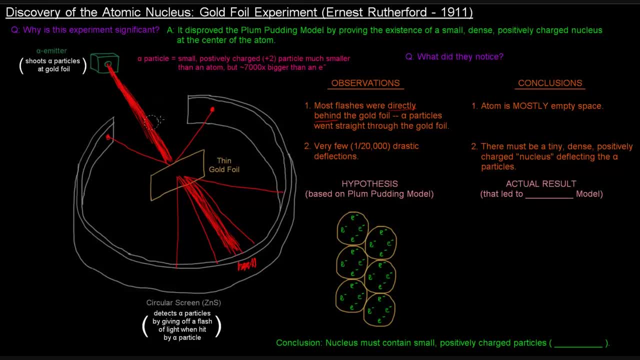 If that's what atoms actually look like, then these particles should go straight through. Why is that? Well, because these electrons, if they're like the dense particles that are contained within an atom, but they're 7,000 times smaller than the alpha particle. 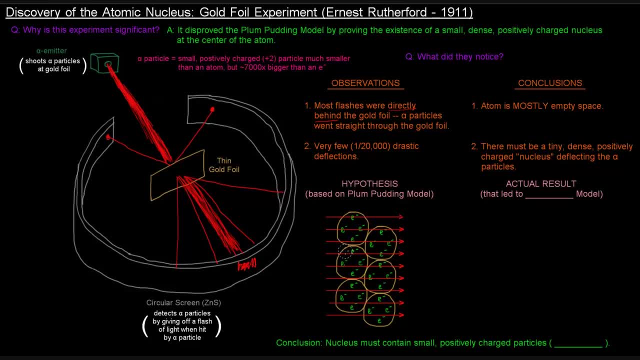 then the alpha particles should have no problem sort of running right through these electrons. It's kind of like the way I imagine it is like a bowling ball being launched at a tiny like poppy seed or like a BB or something right. 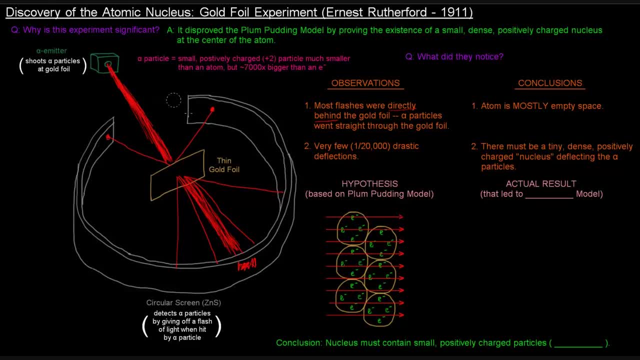 If you think about the alpha particle being the bowling ball and the electrons being 7,000 times smaller, like the size of, like I said, a little BB or a tiny, tiny ball, um then those the tiny ball is not going to deflect the bowling ball anywhere, right? 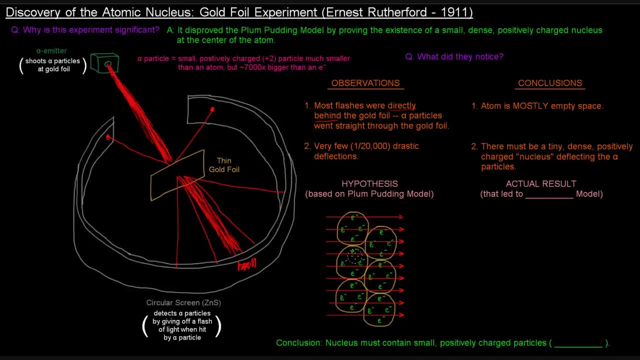 So most of them should go straight through. So that was the hypothesis, because it was based on the plum pudding model. So when they saw that there was deflections like this, where the alpha particle would actually go backwards in the direction that it came from, 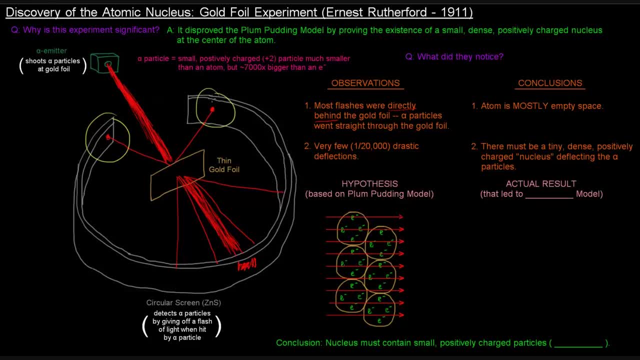 that was pretty crazy to them. That was pretty crazy that this, that these, that this situation even happened. So what that led them to believe is that there must have been something in the atom that was dense enough and large enough to deflect the alpha particle backwards. 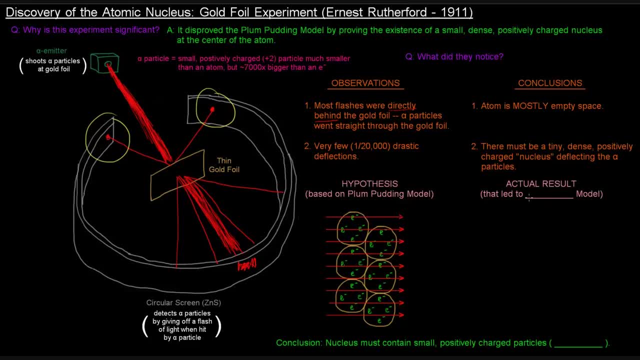 So the actual result led to what was called the nuclear model, which we'll actually talk about in the next video. Um, but I'll kind of show what the result looked like here. Okay, so just a moment actually. So they reasoned that there must be something tiny, dense and positively charged at the center of the atom, like this: 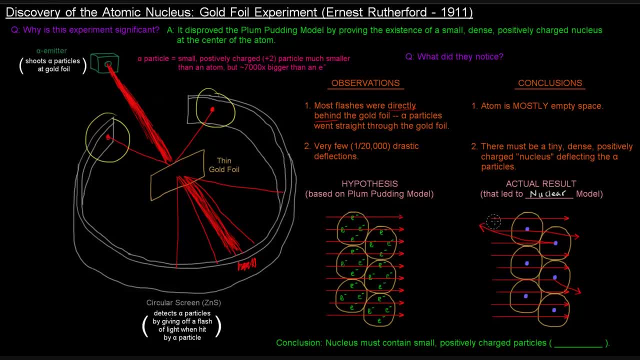 such that the the alpha particles would. the alpha particles would come in and most of them would go straight through, but there would be some cases in which the alpha particle would come in, bump into something tiny and dense and deflect off like this. 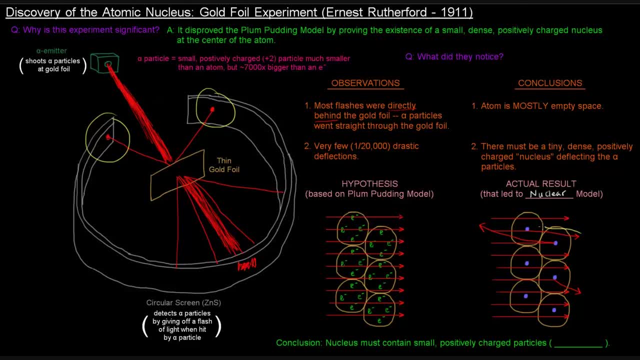 Maybe I should do that in a different color or just circle it See how this is kind of directed off off course, right, And this one, if it, if it hits the right way, it can actually be directed backwards, right. 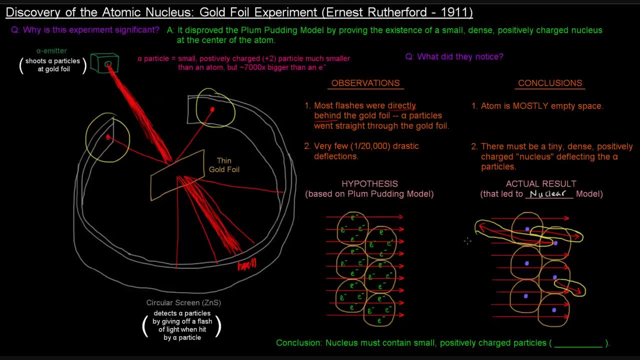 Or this one kind of being knocked off course, Since there were so few of these drastic deflections that that led to the idea that it must have been pretty small. It's been a tiny, tiny, dense um situation in there.